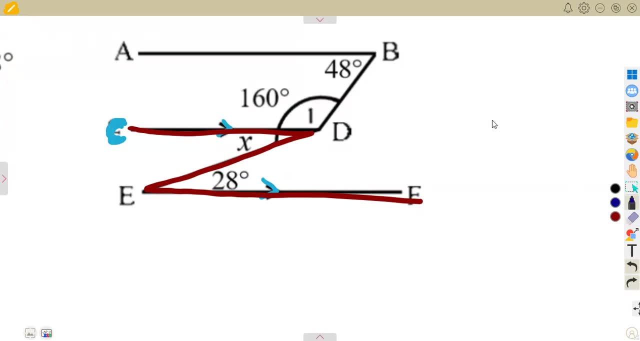 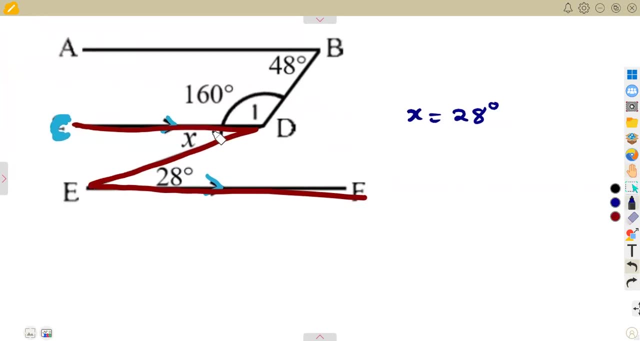 So meaning to say in this part that we are seeing our angle. X is equal to 28 degrees. See where the X is. This is our X here. This is where our X is. So X is equal to what? 28 degrees? We are talking about what? 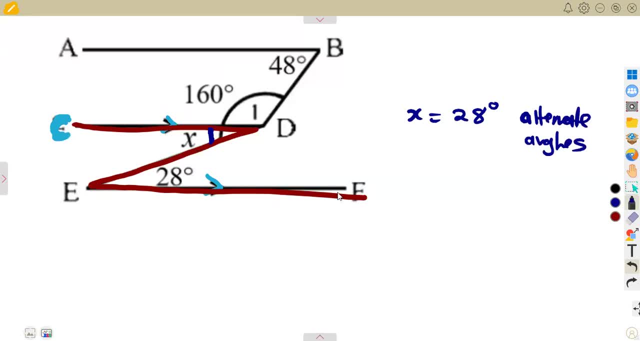 Alternate, alternate angles, That is, alternate to these 28 degrees. So these two they are equal. So X is equal to 28 degrees. But I want you to be careful how this is given before. Are you seeing the 160 degrees? 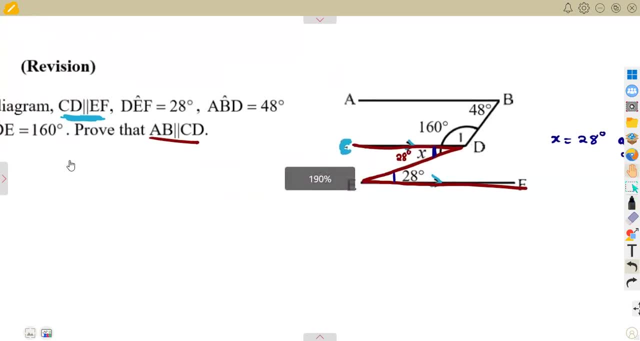 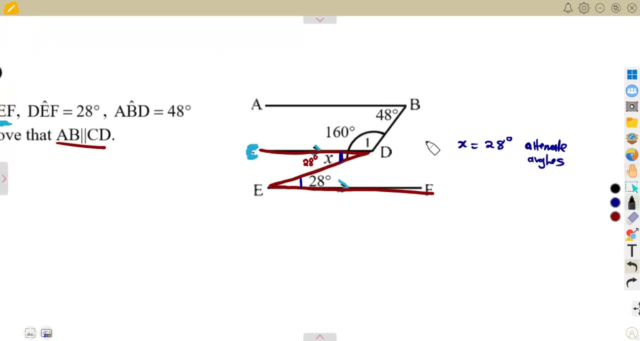 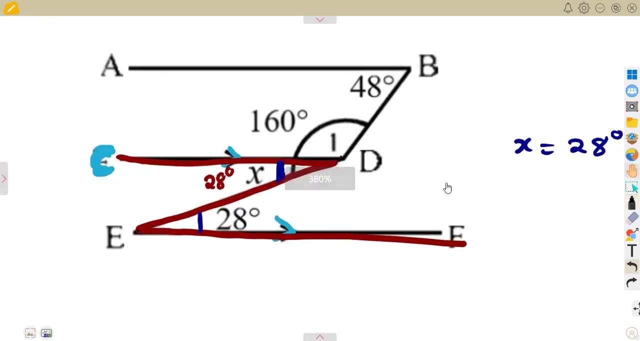 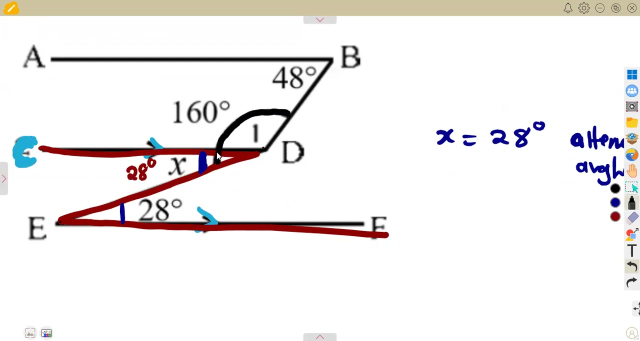 It is the wall of this angle. Let's go back here. Let's go back here. 160 degrees, It's B D E, B D E. from B to D to E. That is the wall of this one. Check, check where it is covering. I want you to be careful about this one, This one from B to D to E: the wall of this one. 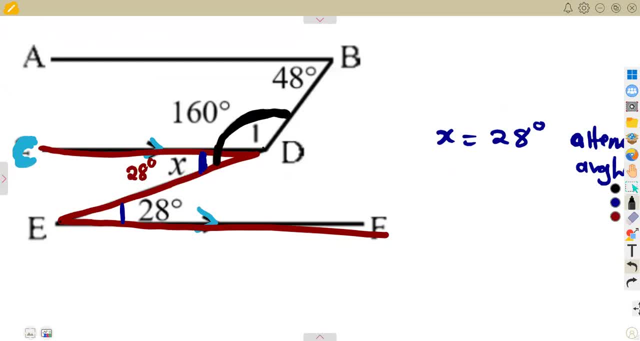 It means it is also covering up, It is also taking up this X. The X is also involved in this 160 degrees. In this 160 degrees, X is also there, which is this 28 degrees. So the question is: for us to prove that these two lines are parallel, we are supposed to use a concept of any parallel lines. 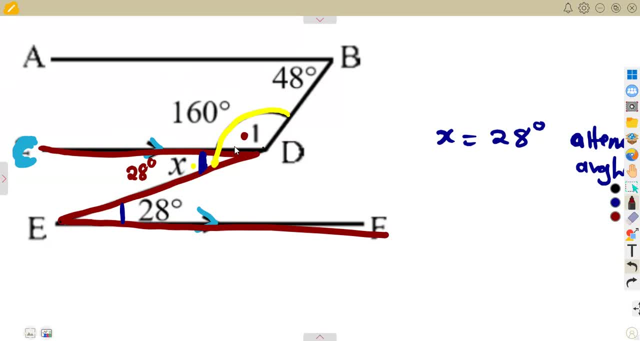 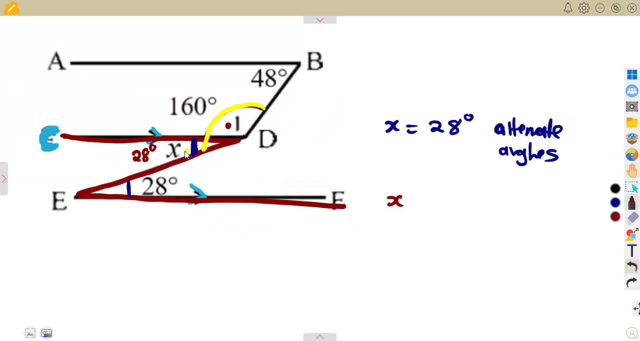 So let's say we can calculate this angle D, Because the combination of what we are seeing, of this, 160 degrees, it is like this, This X that we are seeing here and also the angle D1 that we are seeing here. together they must add up to 160 degrees. 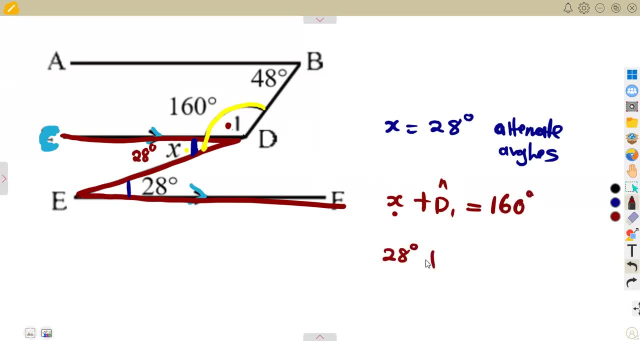 And we have got our angle X. Remember, we said our angle X is 28 plus this angle D1.. This is going to be 160 degrees, So we can transpose the 28.. We are now solving an equation, So that will be a negative. 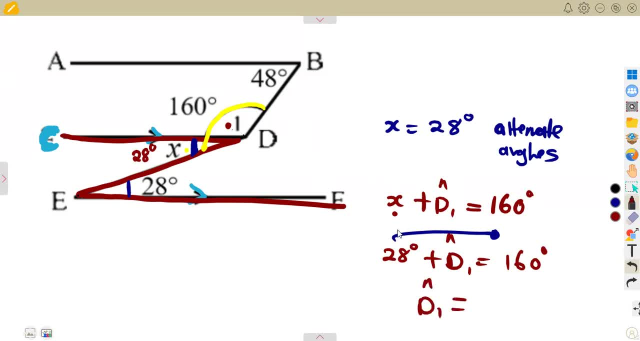 After jumping this equal sign, remember the moment that you get it to the other side of the equation. the sign changes, So that will be a minus on this side. So we are going to subtract the 28 degrees on the right hand side. 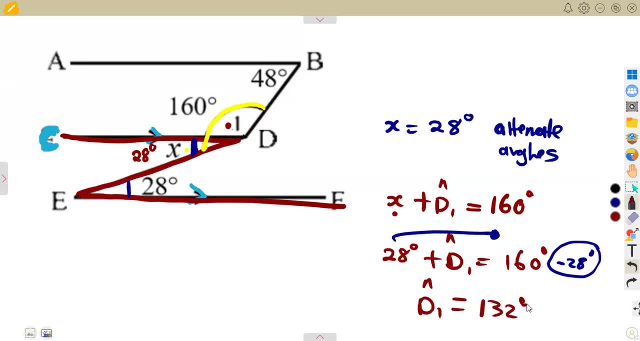 So that means we are having 132 degrees as our angle D1.. Meaning this angle here, D1, D1 is this part, This is the part that I am referring to on our diagram, this one, This is our D1, the part of this angle, the piece of this angle, this one. 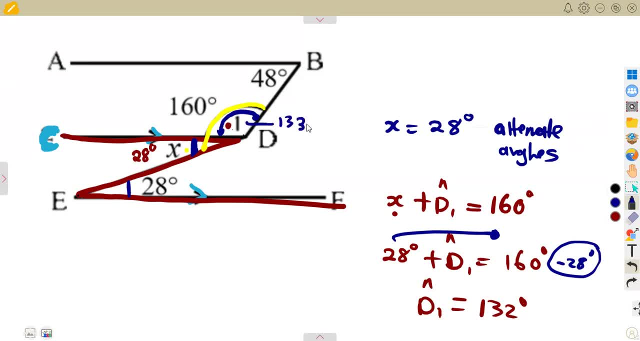 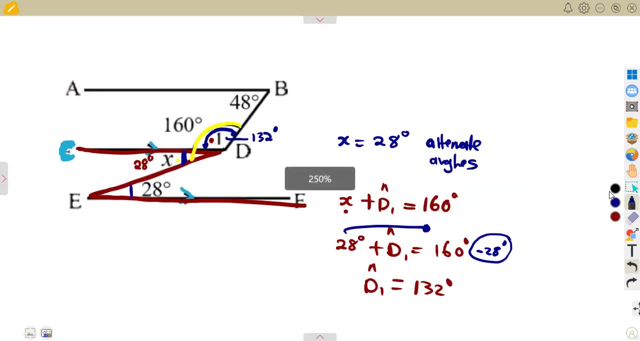 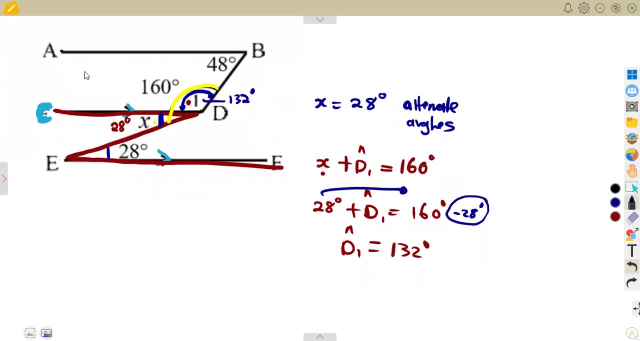 This is the one that we calculated and it's 132 degrees. This is 132 degrees. So now that there is this angle here, that is inside of these two, because, remember, the question is we are supposed to prove, remember that A, B and C D are parallel. 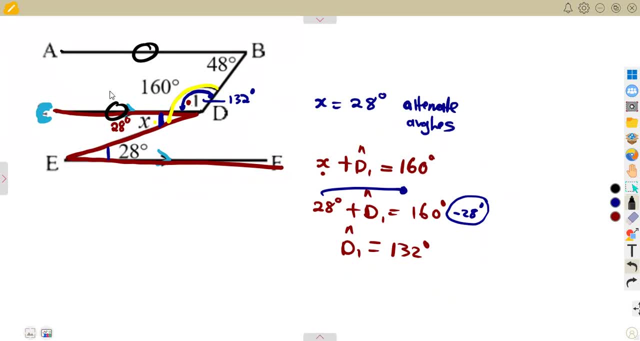 So the question is, if, let's say, these two are parallel, what is that? we know, We know that core interior angles, these angles inside of parallel lines, they are supposed to add up to 180.. So if I am to add the angle D1 and this angle B here, I'm supposed to obtain 180 from the core interior angles. 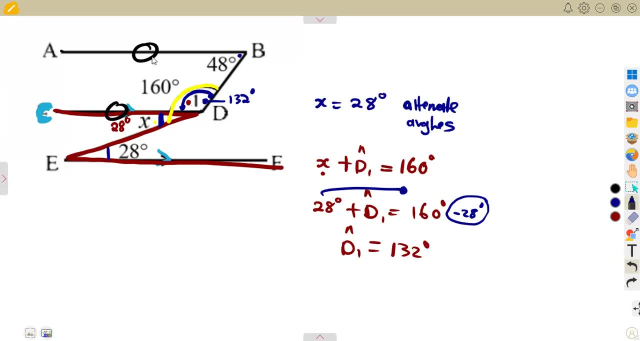 If not, then these lines are not parallel. They are not. So in this case we want to prove: okay. so let us add: angle B plus angle D1 must be 180 degrees. So what are we going to have? Angle B is 48 degrees plus angle D1, which we calculated here. this is 132 degrees. 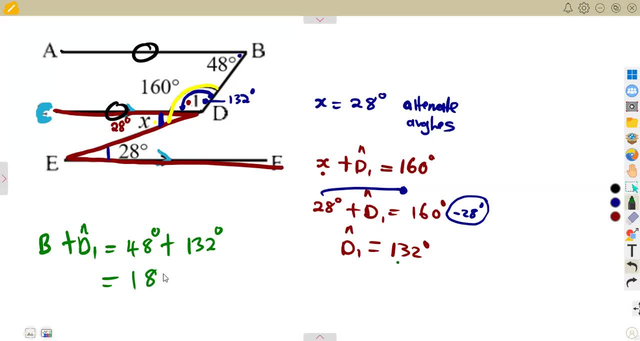 So if you had to add these two, we are obtaining 180 degrees. By obtaining 180 degrees From these two angles, it's not just ordinary, no, It's impossible that you add these two angles, you get 180 degrees. 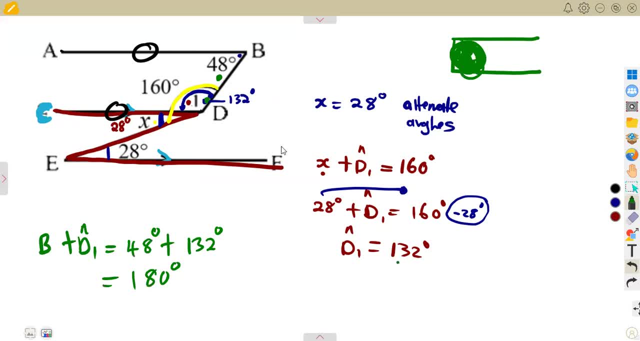 On a normal line. it does not exist like that. It can only exist if these two lines are parallel. Not all lines can do that, Not every line can do that. No, It's only if the lines are parallel. So therefore, this is an indication that AB is parallel. to what?